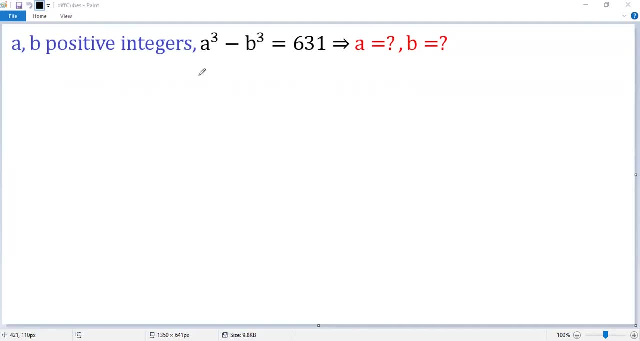 How to solve the Dirac-Fenton equation. Let's check if 631 is a prime number or not. Let's calculate square root of 631.. It is approximately 25.. Next release all prime numbers less than 25.. They are 2,, 3,, 5,, 7,, 11,, 13,, 17,. 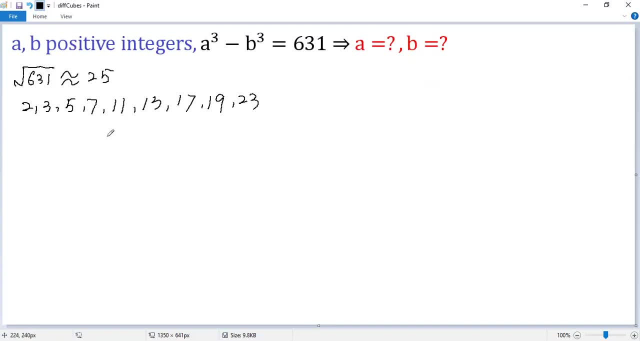 19, and 23.. Now one by one, to check if they are factors of 631.. It turns out none of them is a factor, So 631 is a prime number. Now we can apply difference of cubes formula to write the left side as a minus b times a squared plus a, b plus b squared. 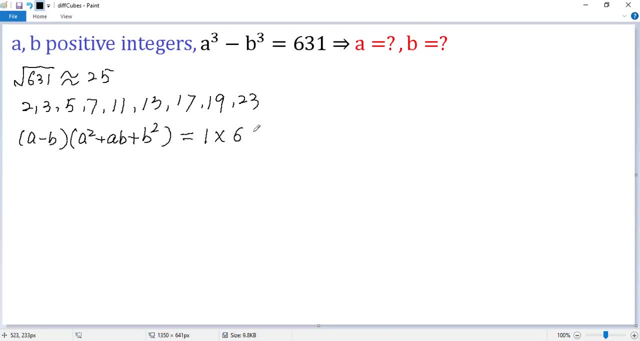 The right side can be written as 1 times 631.. Please note: both factors on the left side are integers And the second factor of course is positive, So the first factor also positive And a minus b must be less than the second factor. So the only possibility would be: 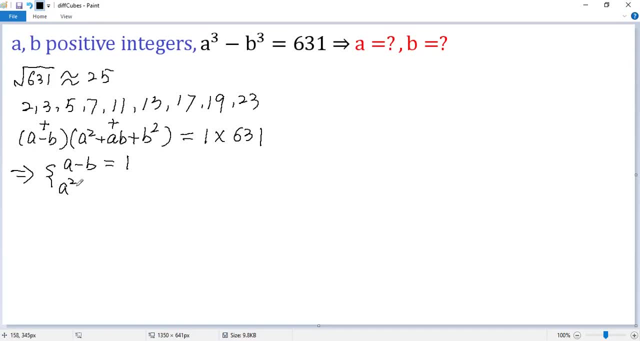 a minus b equals 1.. and a squared plus a, b plus b squared equals 631.. Denoted as 1, that's 2.. From 1, we can solve a equals b plus 1.. Denoted as 3.. Now substitute 3 into 2.. 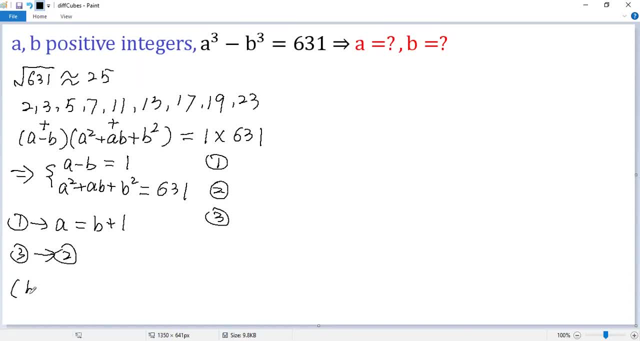 So we get a squared, so b plus 1 squared plus a, so b plus 1 times b plus b squared equals 631.. Expand the left side so we get b squared plus 2b plus 1, and then plus b times b b squared. 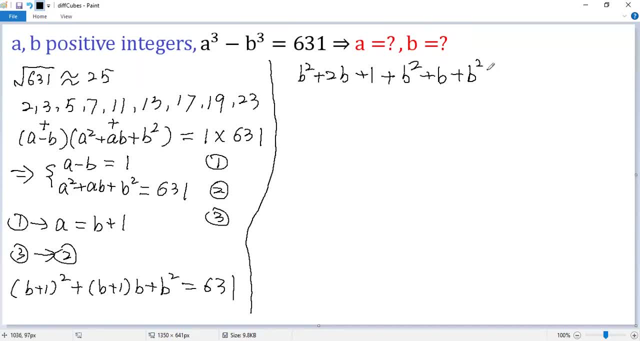 1 times b, b and then plus b squared equals 631.. 1b squared 2b squared 3b squared 2b plus 1b 3b, Both sides subtract 1, so we get 630.. Both sides divided by 3, so we get b squared.